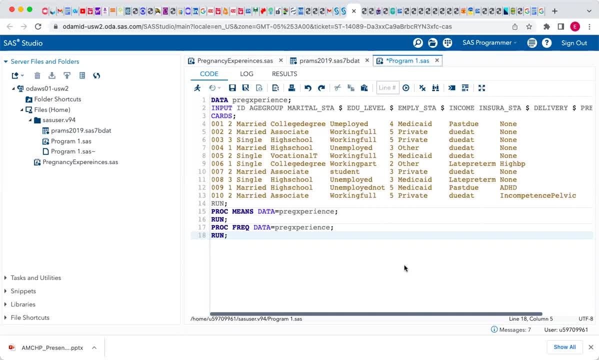 because I'm trying to analyze data for my dissertation. So let's get a new page to start our data, to start this data analysis section. So you go to new on the left-hand side of your SAS software, You see, and you click it new. Then if you're importing data, 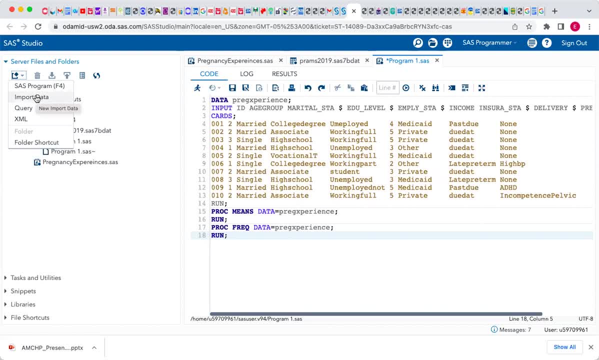 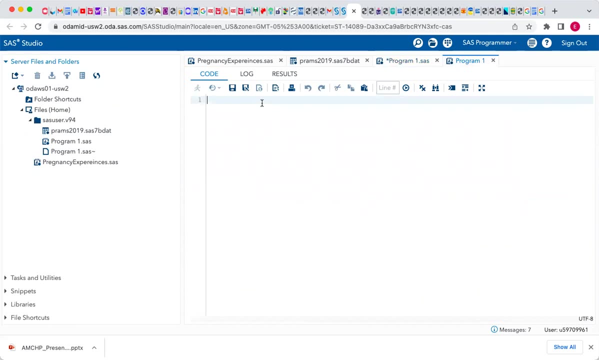 you click on import data. If you already have your data Excel spreadsheet, But if you don't, you want to put it manually on the software, you just click on SAS program. You click this and it creates a new page. You see the blank page. So this is it. So let's. 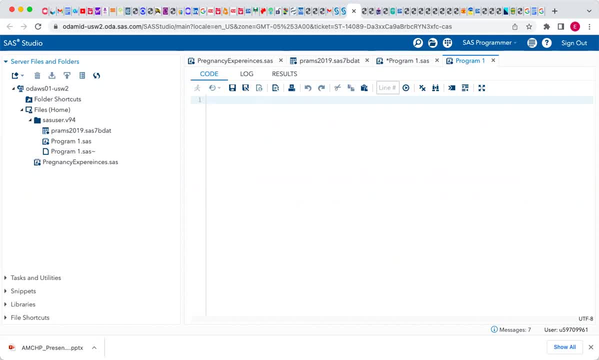 start for beginners. So you start by saying data and you call your data any name. So let me say that I call my data, my data, any name. Let me see You call it any name, That's it. So whatever data you're doing, you call the name. That's what you're going to do. So you put your semicolon. 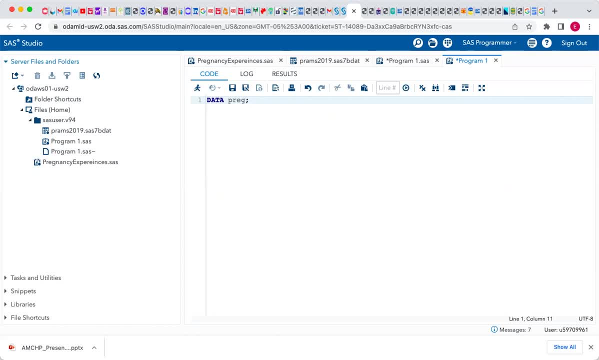 Do not forget to put a semicolon. If you don't, when you run the data it's going to show error. So we go down and you type in imputes because you want to put in your variables, So imputes comes. 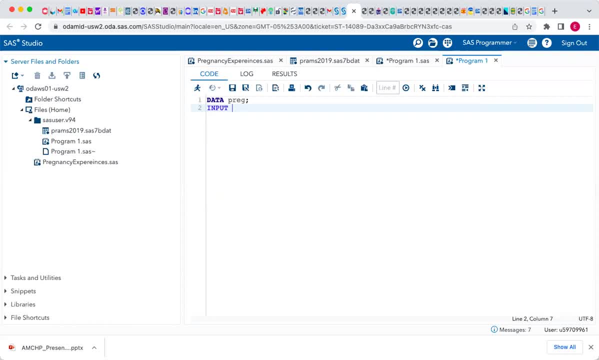 with variable. So let me say I mean I'm using two, three participants, So with their names. let me click names. Normally we're not supposed to have names on data, We're supposed to create ID for them, But let me just use name to make this easier for you to understand. So name. 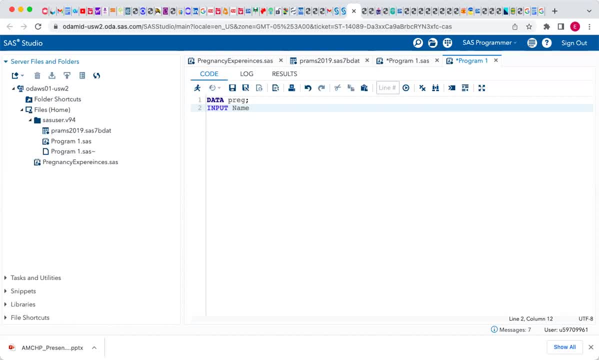 since name is a categorical data, I'm going to put a dollar sign because it's not numeric. Then we have age. We're not going to put a dollar sign because age is numeric, It's a numeric variable. Then we'll look at education. 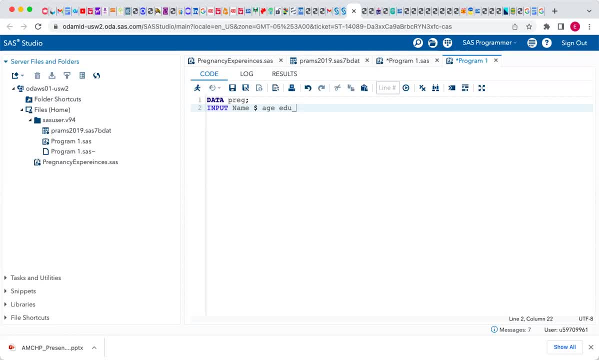 level. Let's say A2 level. I don't need to spell it out. Let's say A2 level, which is education level. Then what a variable will be? Okay, We're looking at. okay, Let's look at. we're looking at- eye blood pressure among males. So we're using 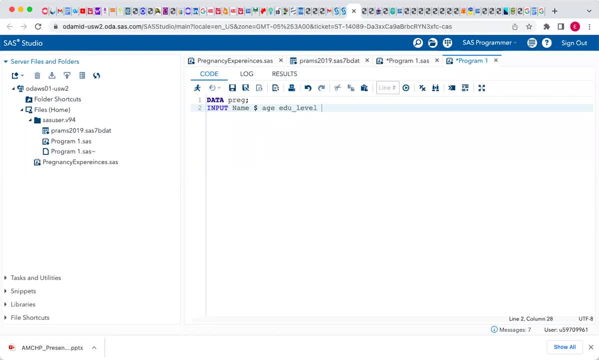 education level and age. So let's use eye blood pressure. So we can do eye blood pressure. Let's say IBP, So high blood pressure numbers. So since eye blood pressure is numeric, the numbers are numeric, We don't need to put a dollar sign at the front. 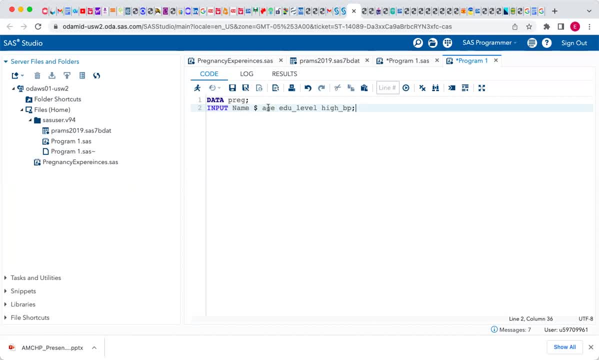 Then we put a column So we're working with how many variables? One, two, three, four, So four variables. So if we analyze this data we should have four variables on our log. Then you click on, you type in cards and you put your semicolon, So cards mean you want to. 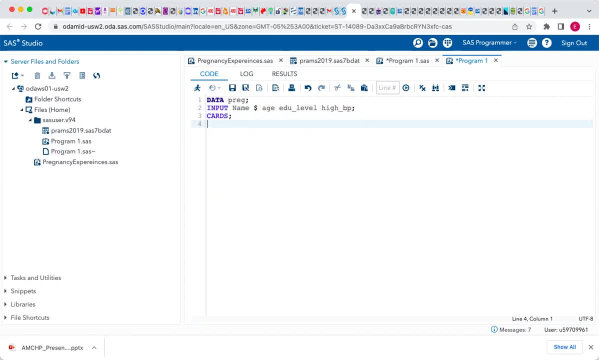 compute your data now. So the name, let's say we have Peter, which is our first participant, Peter. then I'll say, let's say Adrian, Then our third participant should be who? Let's say John, John is our third. 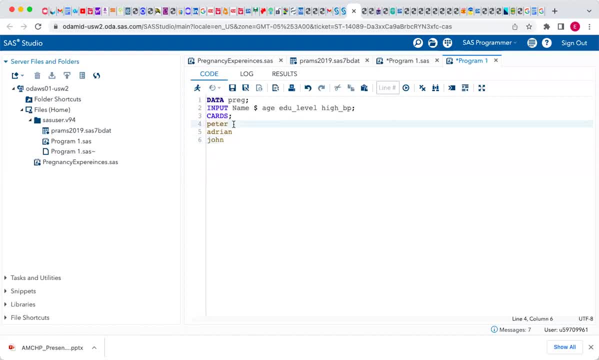 participant. So for John, let's say John age. Make sure you use your space, Do not use tab. You won't get your roles. So we use a space. Is age is what Let's give John age: John 40 years. Then let's give Adrian his space. Adrian is going to be 50.. Oh, you see our column. 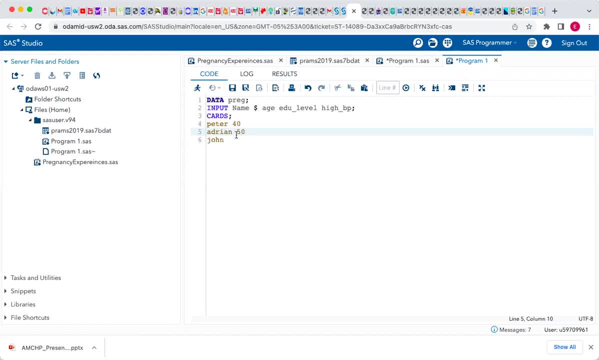 with Peter and Adrian on. age is not the same, So we have to shift the 40. So age needs to be on same column. Okay, So let's move to John. So, John, we're going to space space to the same column. 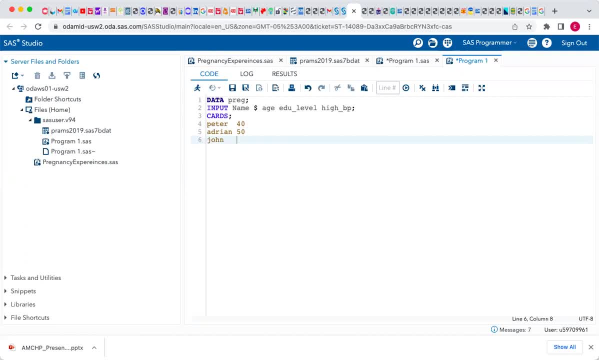 And let's give John John 55 years of age, Then we go ahead After age. what do we have? Education level. So space education level. Let's say Peter is high school, So we put in high school. 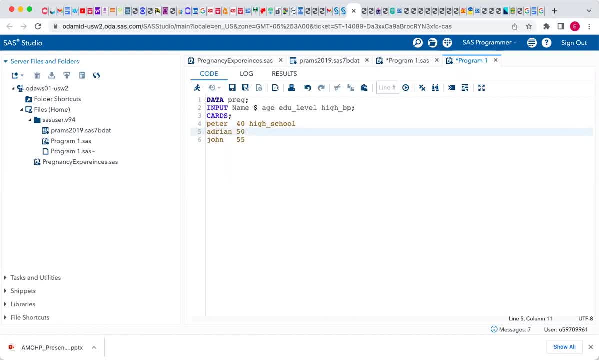 And Adrian high school as well. We put in high school. Then John, let's say college, It's my college degree, So we can just say college. Then after that we go back toLP numbers. So for Peter, let's see if Yeah, has high BP number. 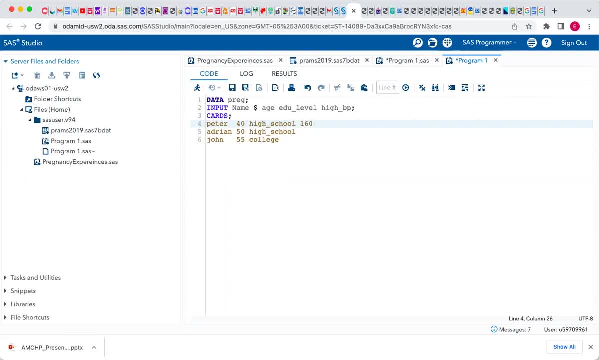 which is 160.. Then for Adrian, let's see he has 100, 55, which BP is high blood pressure, because we know our normal blood pressure is 120 and below. So let's say John, age within 65.. say john, john has a normal blood pressure, numbers 119. 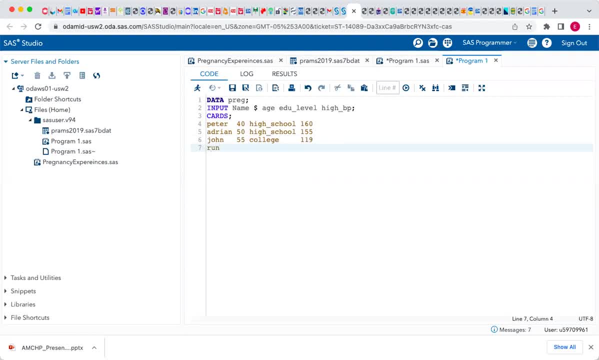 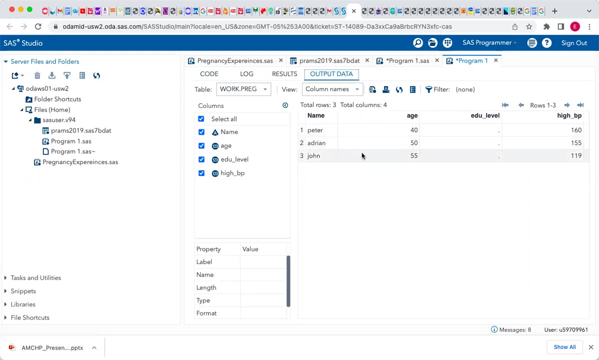 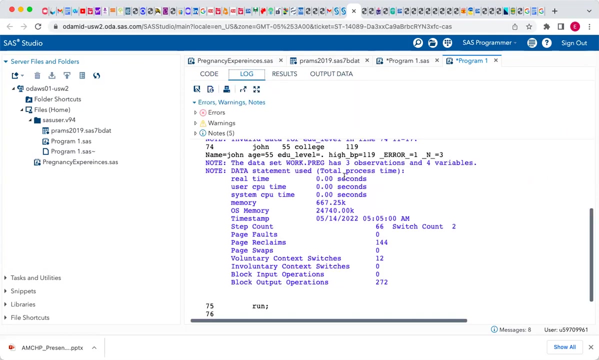 then you enter, we run. remember to put a semicolon before you run your data. so we're not. let's run this data, good job. so when we run this data, this is our input. so let's come to the log. so the log should tell you that we're having what? three observations. three observations means: 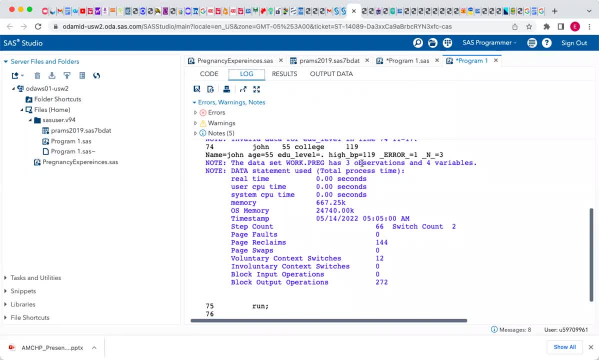 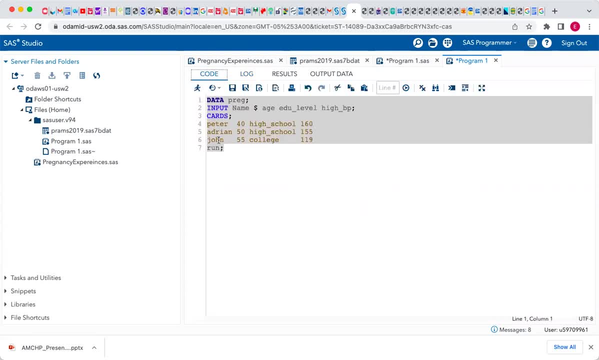 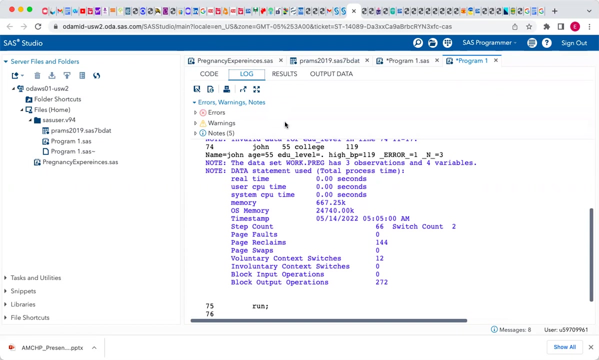 right. here is three, where my cursor is: three observations and four variables. three observations mean three participants, which is what we call here. so three, one, two, three and four variables is our the name, age, high school and what cst. so if this log is correct, there is this is there is no error, so you're good to go. so we have that. 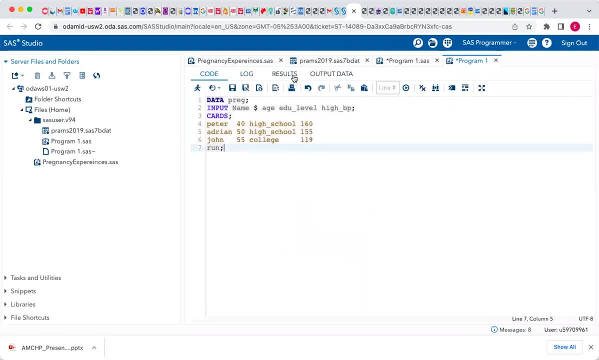 so this is our data. we got that and our observations are good and this is our output and this is what it looks like. so we want to run frequency to know how many number of participants have high blood pressure and how many does not have blood pressure pressure. With this, you can do that to participants who have high blood pressure, So let's run. 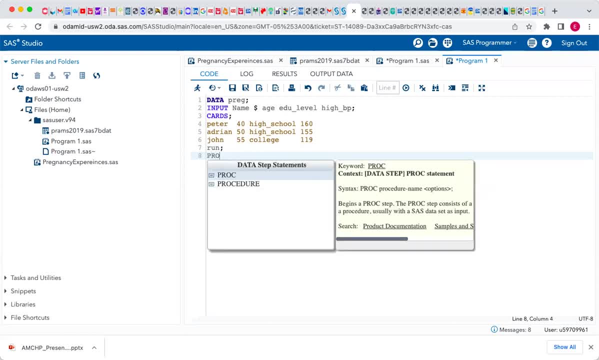 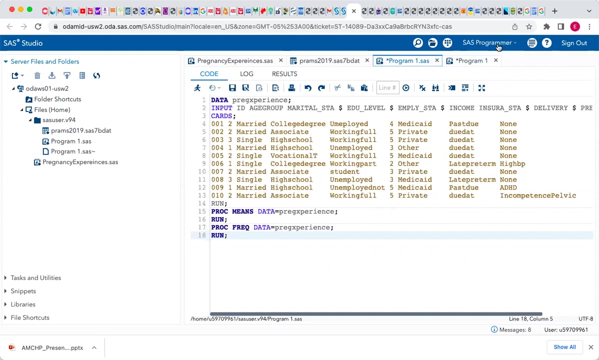 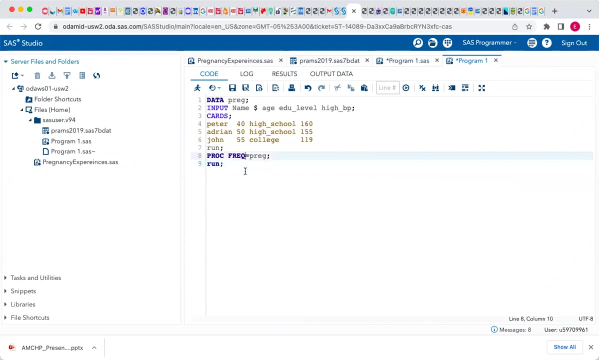 So you do PROC FREQ, PROC FREQ, That is the frequency, PROC FREQ, and you put in the data PROC FREQ equals to FREG. You put a semicolon and you run Ok, So PROC FREQ equals to. 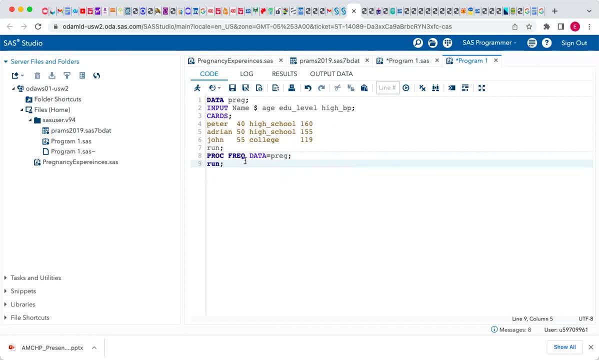 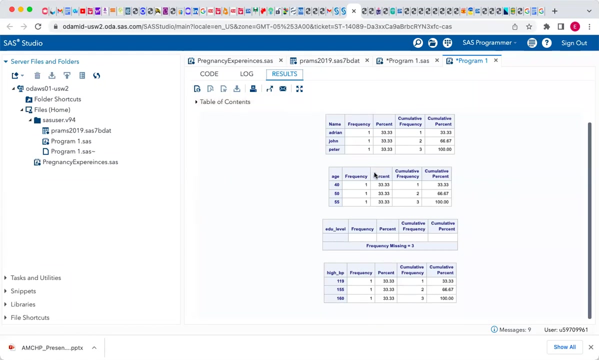 preg. So preg will want to see frequency. Then you say data preg. which is this right here? you bring it down here. That is what it looks like. Put any different data name, you're going to have error. Then we run this. So we get our data. So, like I said, frequency table. 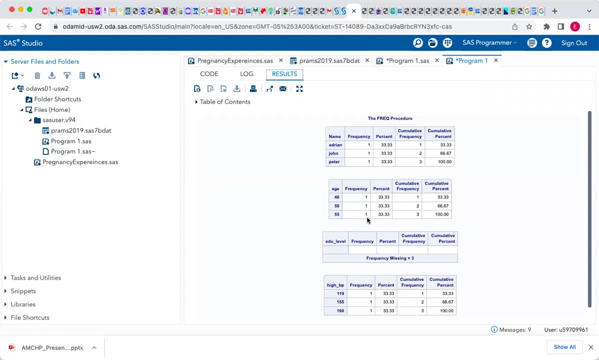 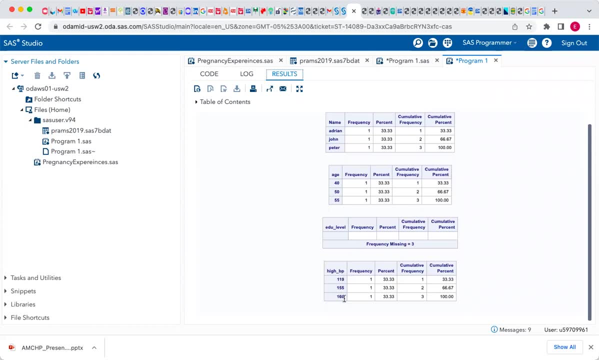 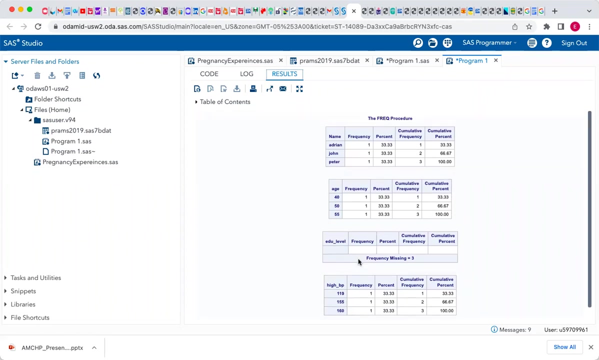 We'll see our frequency. So I have low pressure. This is what our frequency table looks like. So you run your data and this is the result: 05 01 01. 01 01 01 01. These is the result you have. 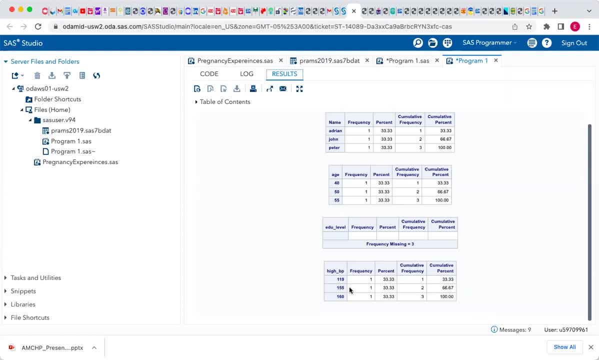 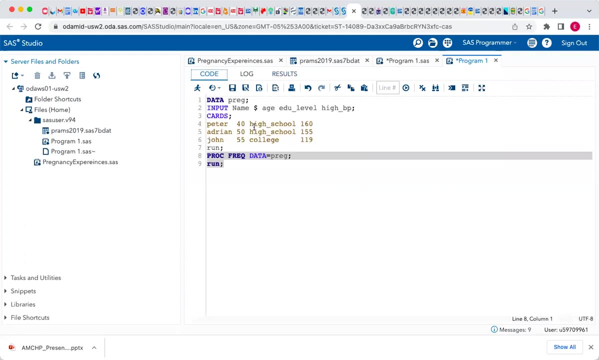 So you can see that for high blood pressure, numbers 1, 19, 1.. I put 1, 19 as one, so it's the same thing. We go back to the code and say I have low pressure, We have 160. 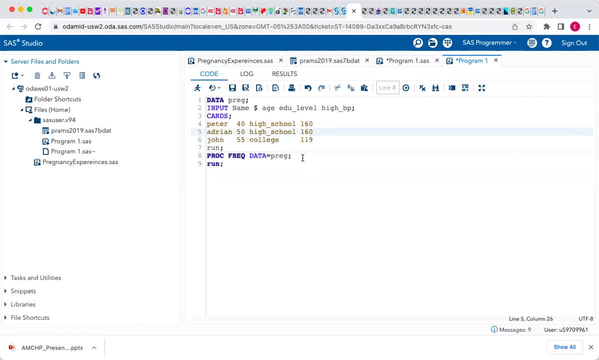 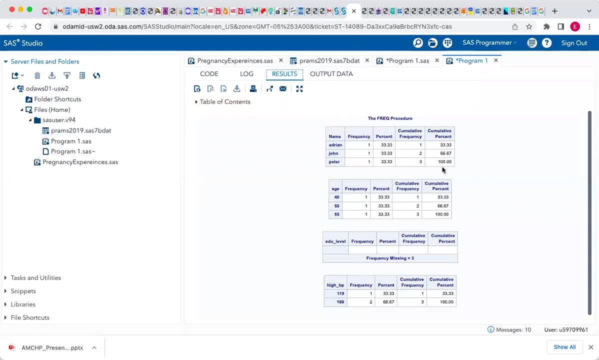 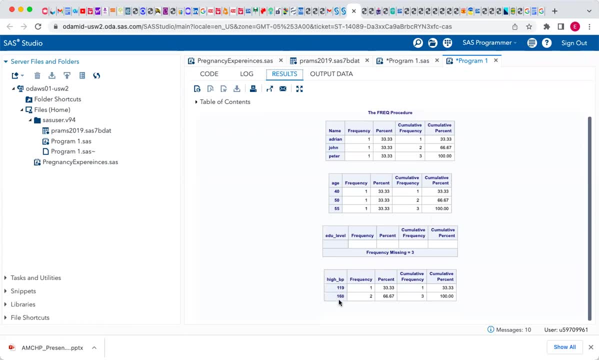 So you see, because we have for high blood pressure, we have two people, which is we had two people who had 160.. So the frequency was two. The 119 is one person. So we have one person. that's for our frequency for high blood pressure. 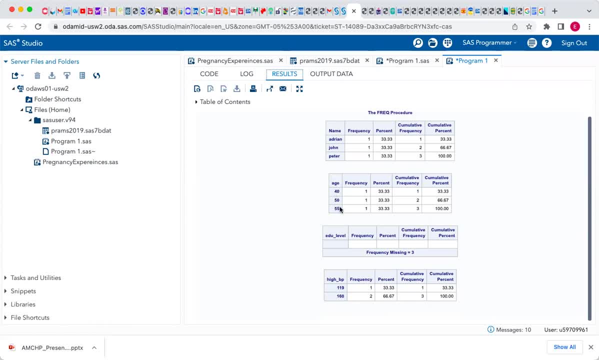 Then our frequency for age, because they all have different age. So 40 was only one person, 50 was only one person, 55, it was just one person. So that's, that is for age and for frequency. for name: we have any name that come out twice. 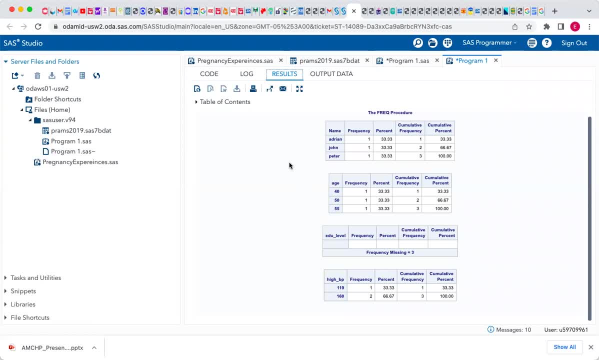 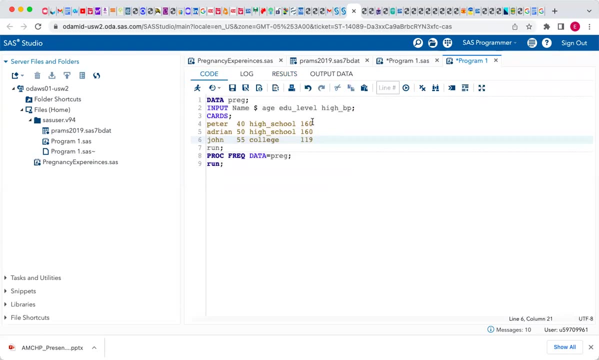 So it's one, one person age. And then for frequency for education level. So we're going to go back see why it's showing a frequency for education level missing. So now we come back here So we need to put Since education level. you see why it didn't come up? because education level is a categorical. 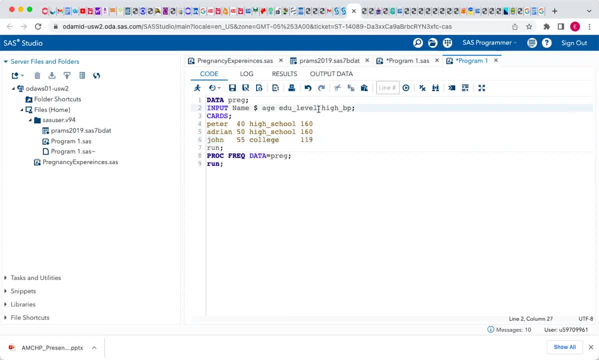 data and I didn't put the dollar sign. So, since education, then you're not going to get your, your, your, your variables are going to be missing If you didn't put a dollar sign, just like the name. I put a dollar sign because it is. 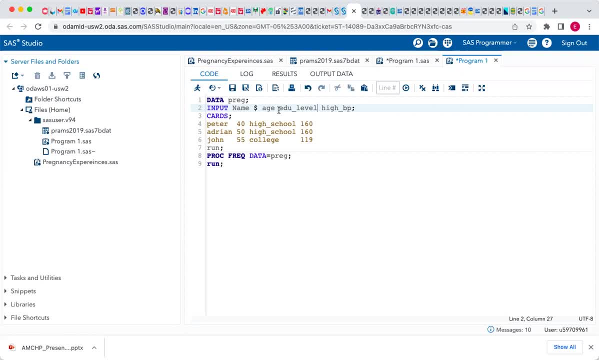 a categorical data. So your age. no dollar sign in front, Because it's numeric data. Your education level should be what? A categorical data, and it should have a dollar sign in front. So now let's run it. we're going to have our data. 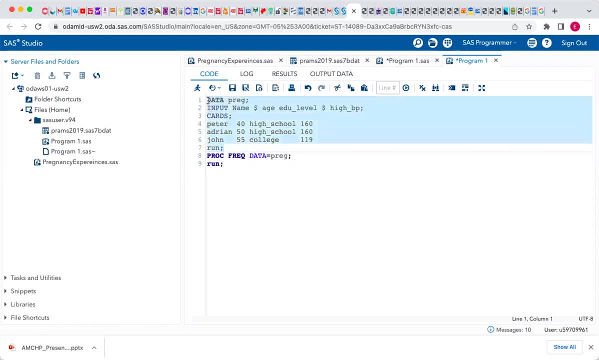 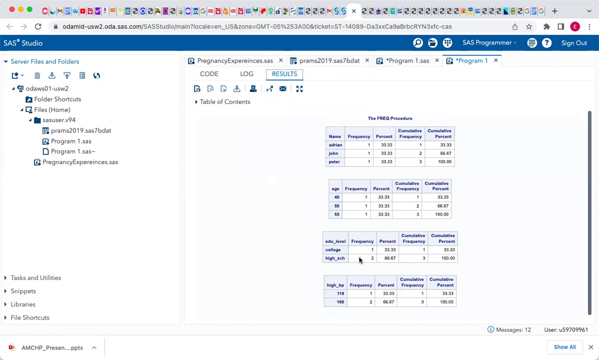 Go back and run first. let's run this data first. run this to have it. then let's go and run our program. We're going to use CROC Frick run. Yay, so we got our education level, you see. 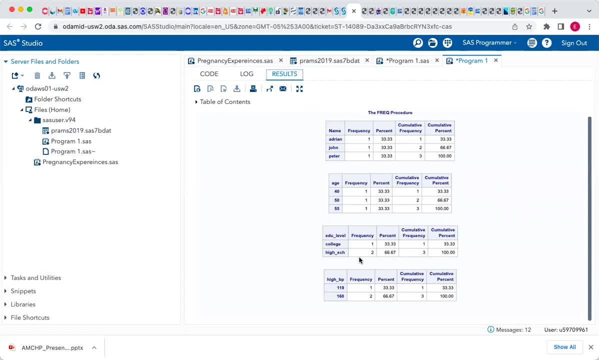 So, whenever you're using a categorical sign, make sure you a categorical variable, Make sure you put a dollar sign in front, because it's not numeric. So, education level: we have one person. frequency: frequency: one person and uh, for high school: we have two people. we have two person for high school. 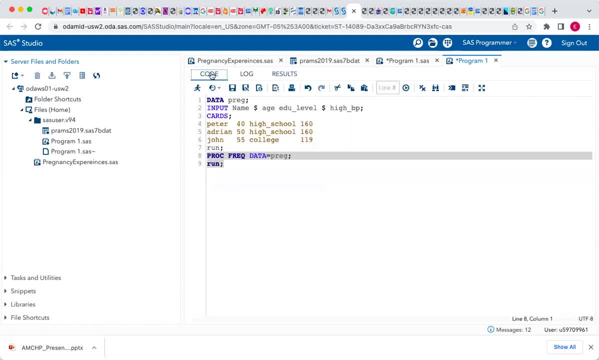 so right now, if you want to run your data and you want to see if education level have an impact in high blood pressure, because on this data we can see peter has a low high school degree and adrian has high school degree and that blood levels are high. so if we want to check if education level, okay, now we run. 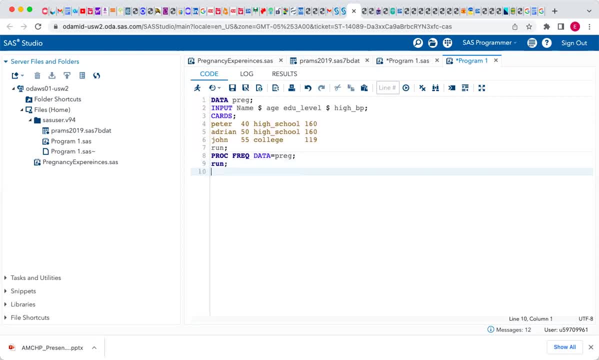 prog free to know the frequency. we can go ahead and run. prog means prog means prog. data equals to preg. okay, data equals to preg, then we run. you can pull craps log. you can pull lowercase, that's fine, okay, so definitely i'm making something error for that not to work. 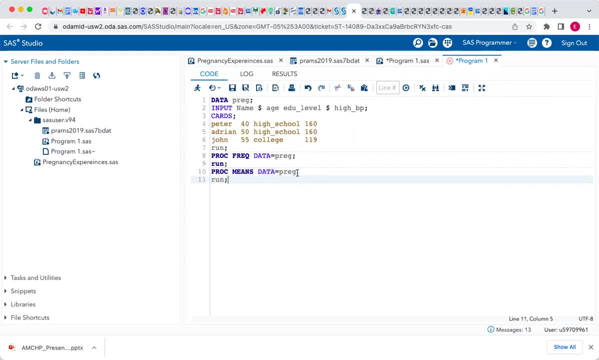 see, i purposely make this error. why? because there is no semicolon in front of prague. so these are the little mistake you don't want to make when you're greater. so let's go ahead and run it again. good, so this is our. what our mean procedures? so this procedure, you see, uh, 12 conservatives right now is strata of a human outer. Houk ambassadors here. let's lipularization return to how tofle. 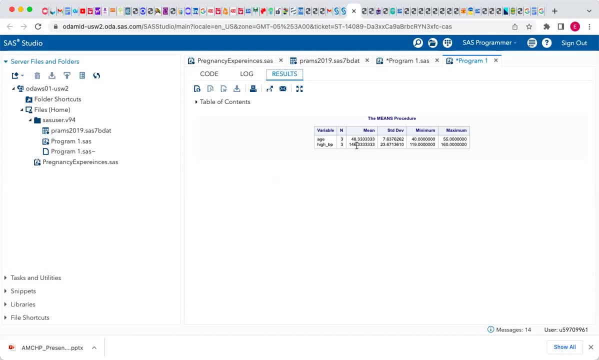 age, the number, we have three people. then eye blood pressure: we have three, three people definitely who reported eye blood pressure. then our means, which goes on with our age, and you see the standard deviation, the minimal and the mass. so this is what you do. go back to code. so this is for.